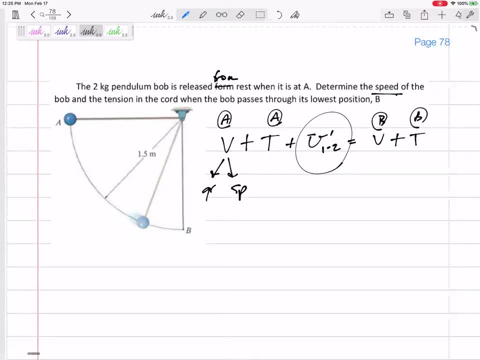 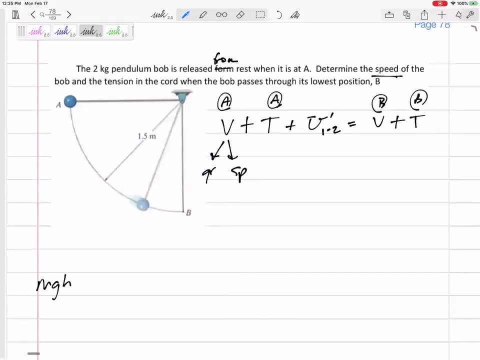 The work is throughout the problem, from beginning to end. All right, so this is what I kind of like to do. There's no spring in here on this problem, right? I probably should just go ahead and and neglected that. It said something about it started from rest. You could go ahead and set. 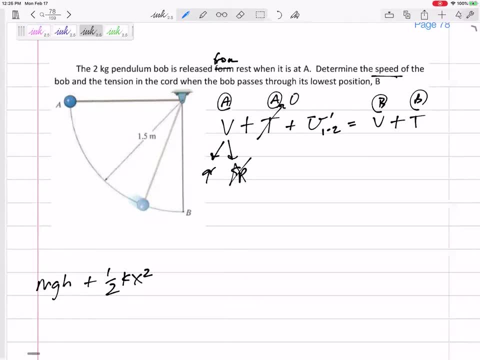 that initial kinetic energy to zero. But if you like to, this is what I like to do. I don't know about you. I like to go ahead and write this whole thing, all of the terms that I could have. Now this might take longer than you know, if you, if you recognize I don't have this. 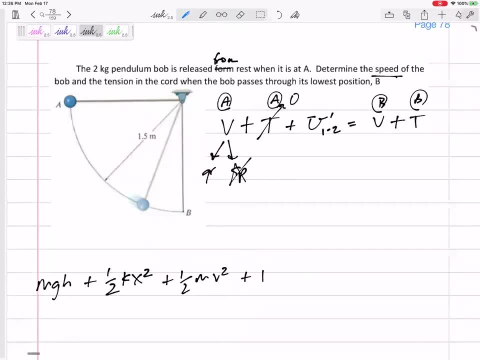 I don't have this, So this isn't necessary, But I like to just write: mgh is one half kx squared plus one half mv squared plus FD. Now I'm going to put FD right here, but it's really integral FDS. 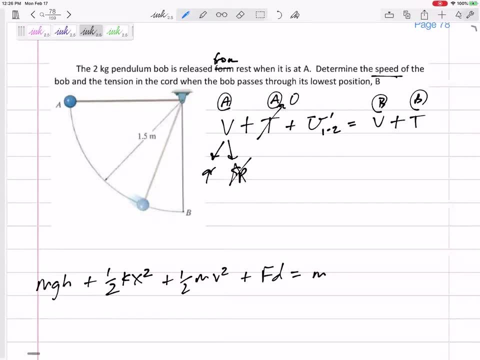 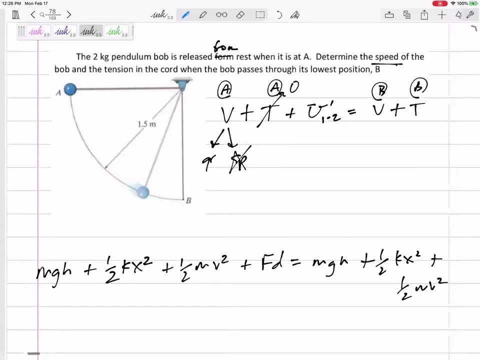 But it's FD if it's constant Equals- mgh, final one, half kx squared, final one half mv squared. So I like to kind of get that long equation. That is my conservation of energy equation. So I, you know, sometimes I'm I'm bad about about going through these motions before I really 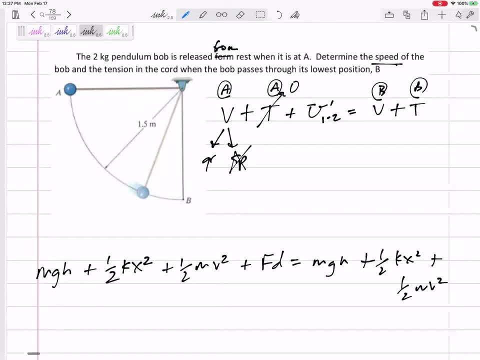 read the problem and really, what am I trying to find? What am I given? But if I know I'm going to use conservation of energy method for this problem, I like to go ahead and write that whole equation and then ask myself: okay now, now I can break it up into like bite-sized pieces. 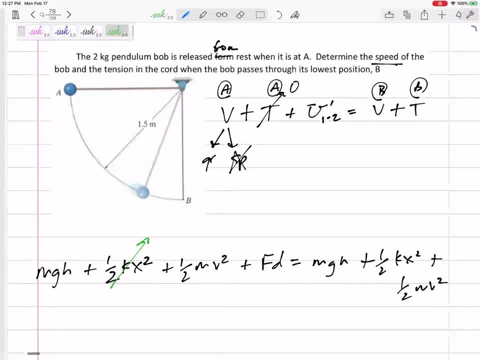 right, A lot of these would be zero. All right, Obviously there's no spring, So there's no one, half kx squared right here. Uh, it started from rest. Yeah, Many, many of these problems will start from rest. So there's no um kinetic energy initially. 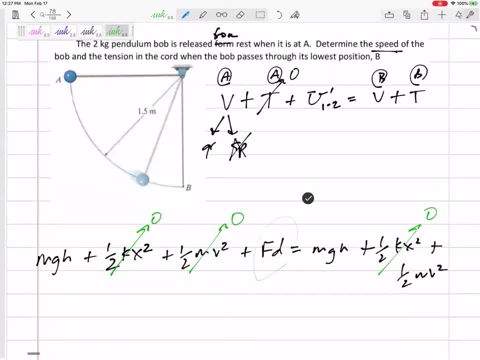 All right, What about this FD right here? So this is maybe a force that's drawn on the figure, just an external force that's being applied, or maybe a cable like that previous problem: a cable, a rope, a tension that is pulling a distance? Uh, there is a, there is a rope in this problem. There is. 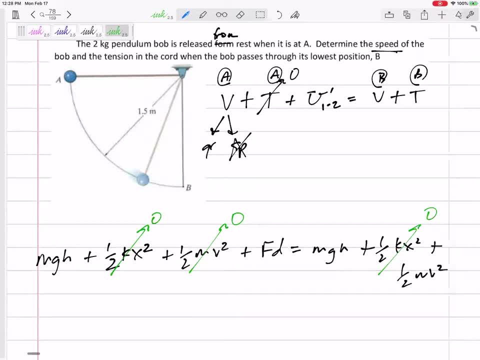 tension in this problem. but you see that that tension is never going in the direction of the displacement, That tension is not doing any work. That tension is not doing any work. Uh, so, so there's no, there's no sort of external force, times, distance for this problem. right, Tension is always this. 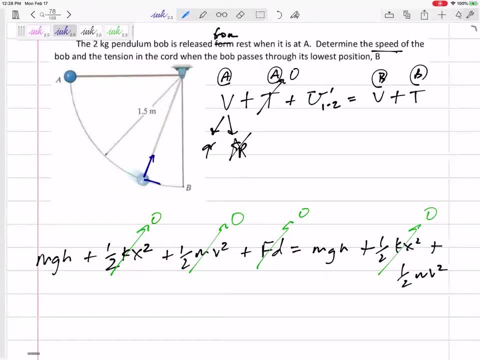 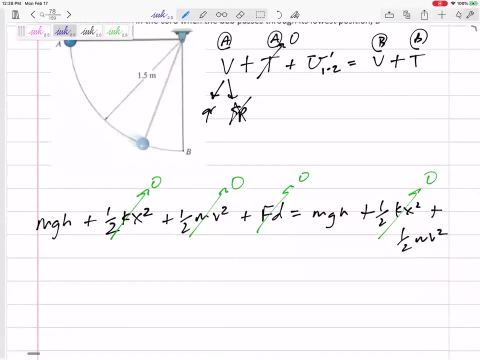 way, but the displacement is always perpendicular to it. What component of my tension is in the direction of my displacement? None of it, Yeah, None of it. All right, So my equation really boils down to: MGH equals MGH plus one half MV squared. And so, if you could go ahead, 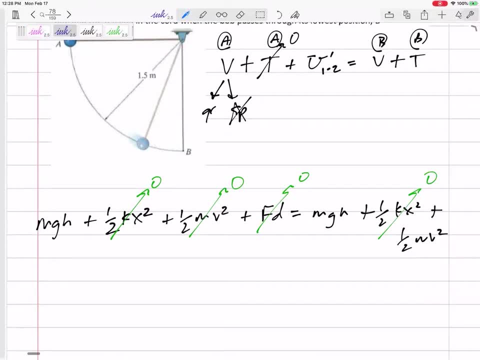 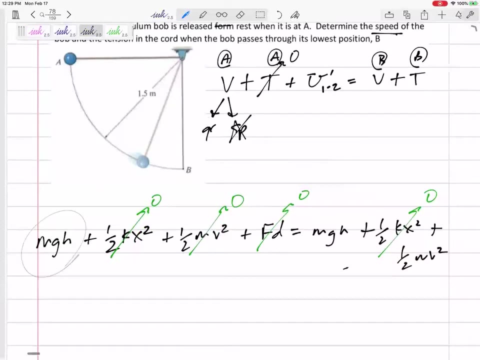 and realize that you could start with that. MGH equals MGH plus one half MV squared. I like to start with the long equation and mark things through. It feels good to kind of put a big X through it, put a zero through it, Okay. So let's think about the MGH initial and the MGH final. 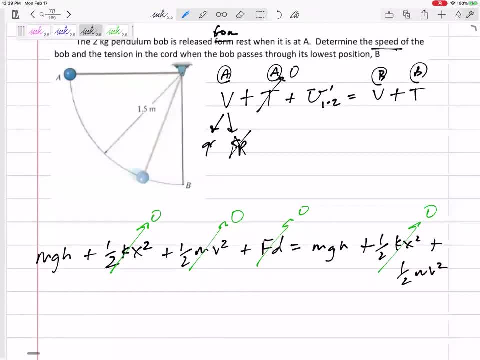 For this MGH you have to choose positive up, but you can choose your ground to be wherever you want to Um. we've got two good options. I think we could choose that to be our ground, Um, or we could choose 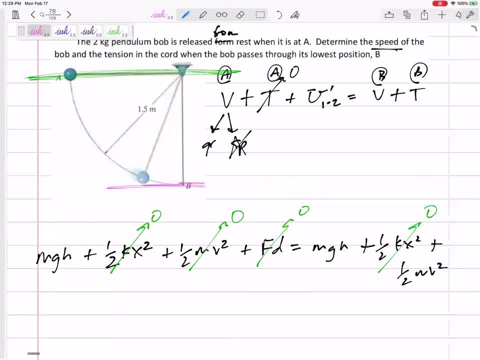 choose that to be our ground. Um, I'm going to use this green line to be our ground. So that means it starts at a height of zero and it ends at a height of negative 1.5.. It ends at a height of. 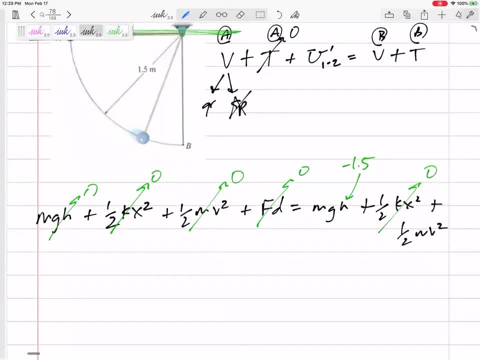 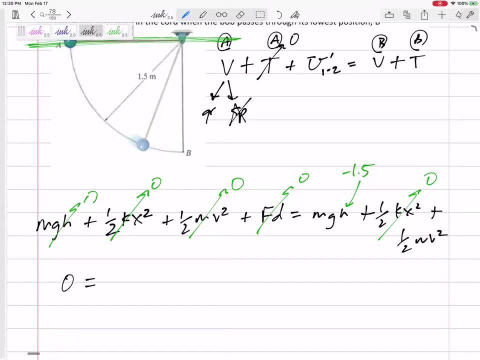 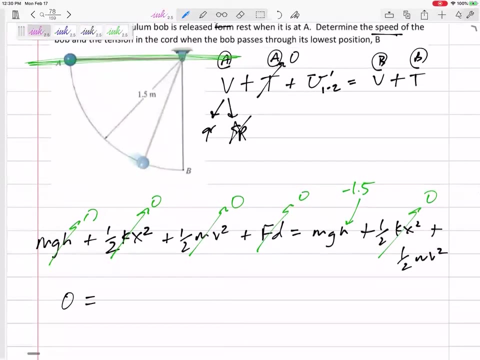 negative 1.5.. All right, So left-hand side, we've actually got zero. Is that okay? Well, we'll see. We'll see What. what was our other option? Let let me just show how this would be the same. I think y'all can. 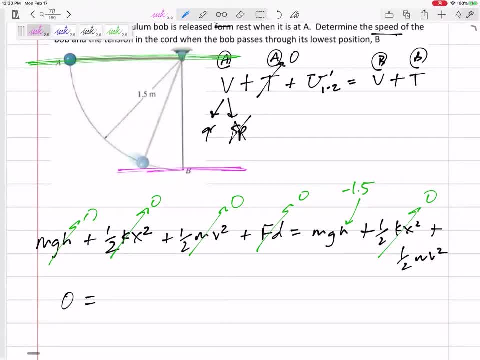 understand how this would be the same If we chose pink to be our uh height, our zero, then we would say it starts at uh 1.5 and it ends at zero. and see how mathematically those are the same right. 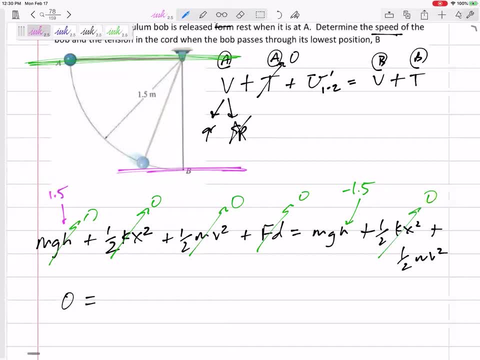 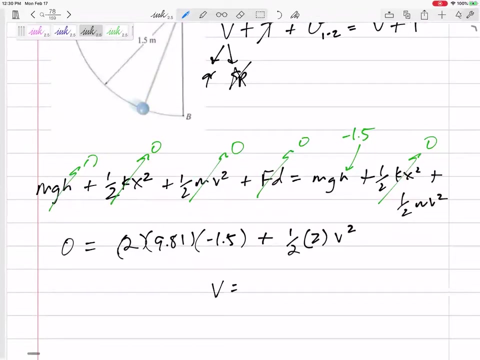 1.5 on the left or negative 1.5 on the right. Okay, So zero equals M. What is our M here? Two, 9.1. height of negative 1.5, plus one half M V squared. I mean that that really became a very simple equation. Yes, 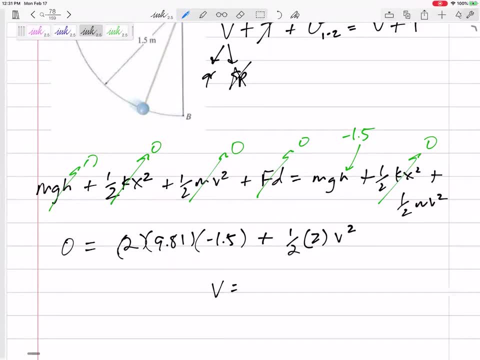 No, no, that is. it's not really acceleration, It's just G. All right, And we've already, we've already defined it going down, So I already know it's going down. That MGH, that G, is just the magnitude of G. So, correct, Do not put. do not put. very important, do not put. 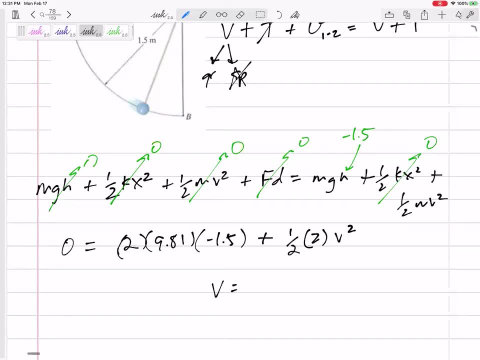 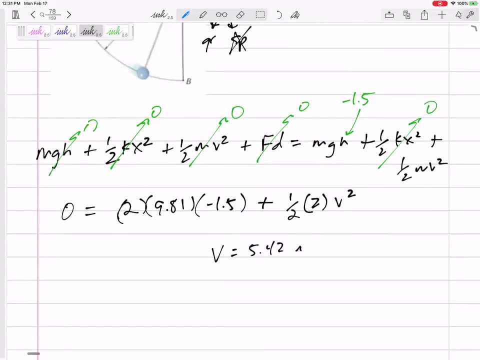 negative 9.81. right there, Okay, All right, So I've got. velocity is 5.42 meters per second. boxed it in. That was one of the things that it asked for the speed. Now it also asked for the tension in the cord. Where was tension? 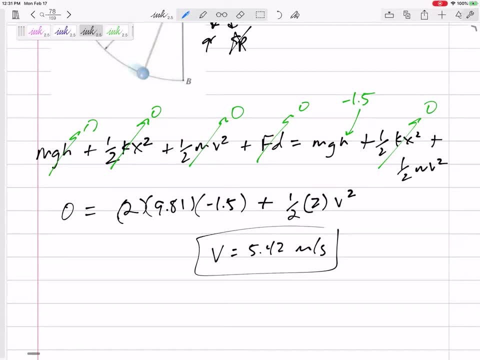 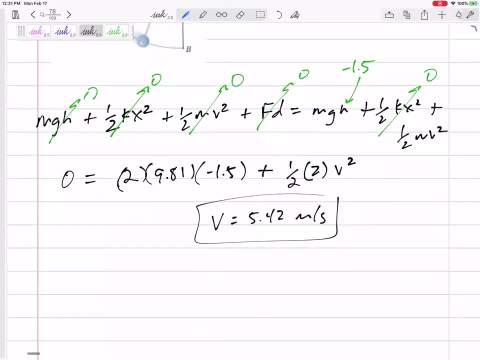 in the cord in this equation? It was not in this equation. It was not in this equation. So I've got to come up with a another way to find the tension besides conservation of energy. All right, So I say that. I say that these problems are like conservation of energy problems. 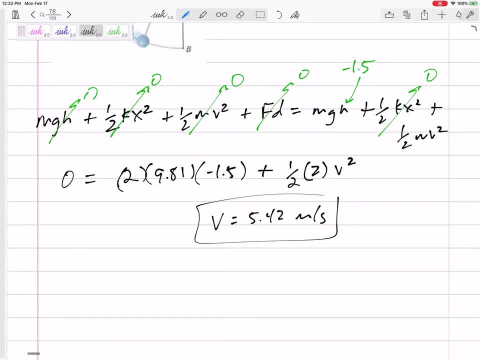 but they might be conservation of energy Plus. I'm about to do a free body diagram to find that tension. So it might be conservation of energy plus free body diagram. We'll do some that's like conservation of energy and then it becomes a projectile. So just because this is problem, 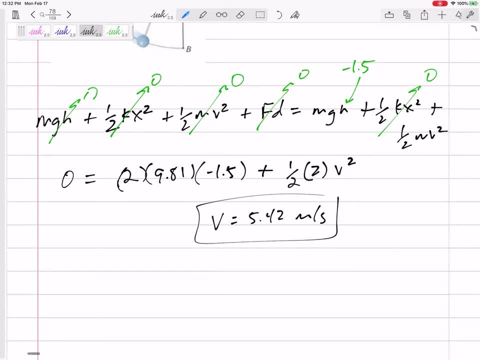 number three: just because this is a conservation of energy problem. you still might use some of our other tools, but kind of the heart of that one is that conservation of energy problem. So I'm going to do a free body diagram to find the tension in the cord at B. So let us, if we want to find 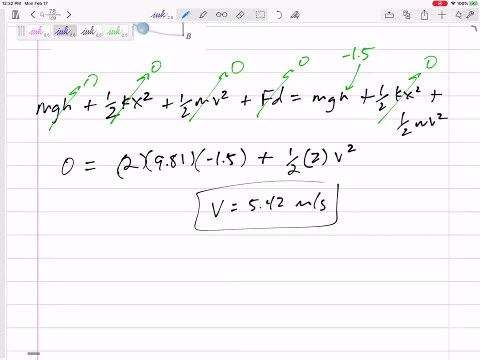 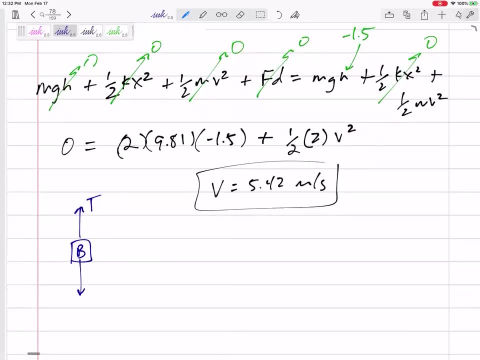 the tension in the cord at B. let's draw this Bob at B and there's tension. What other forces are acting right here? Mg, All right, And I think those are the only forces right there. And let's sum the forces right: Tension minus two: 9.81.. 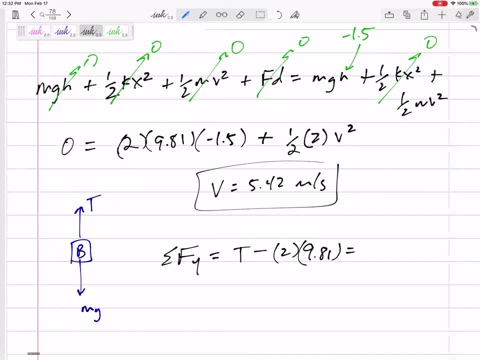 Equals zero. It really is, ma, And is it accelerating in this direction? Is it accelerating in this direction? Should I set the signal to zero? Do you think the tension is just zero? What is this? 18.6.. Or what is that 19 point? I'll give you a hand, It's not. 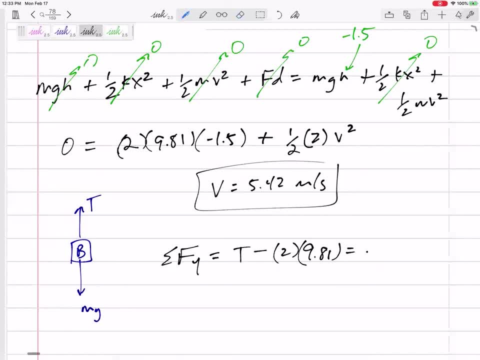 Is it accelerating in this direction? Yeah, Yeah, It is accelerating in this direction Because it's in a circular path. Don't forget about normal acceleration. Don't forget about normal acceleration. In fact, I probably, instead of saying oh, it's accelerating in this direction, it's accelerating in this direction. 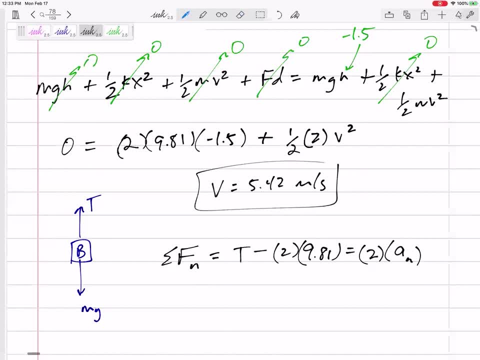 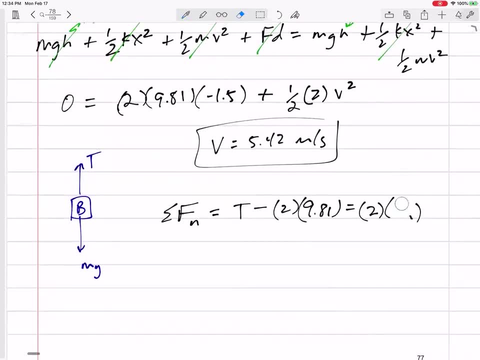 If I summed the forces in Y, I should have said: if I summed the forces normal, you would have recognized that and realized that Don't forget about normal acceleration when things are traveling in a circular path. So this is V squared over. rho, Do I know V Listen up At this instant 5.42.. 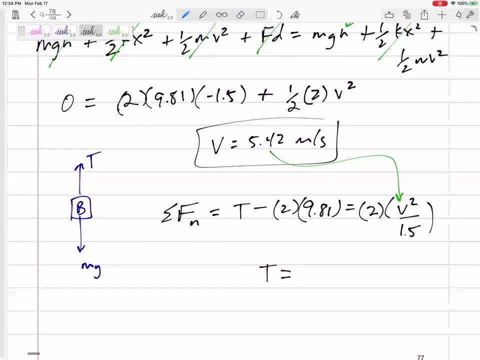 So at this instant, and this is the only the tension at this instance it's changing because the velocity is changing And that free body diagram would change. Tension would be equal to 58.9 newtons, 58.9 newtons. 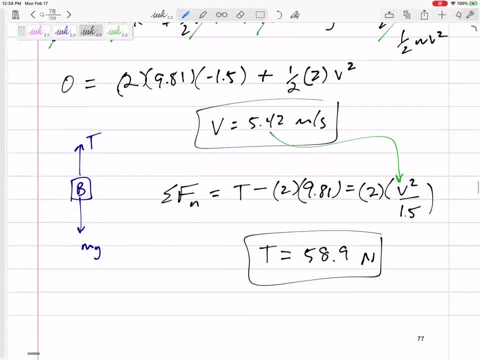 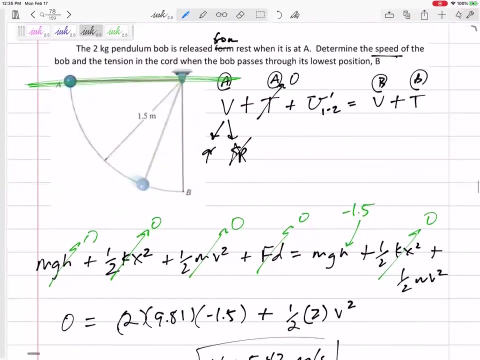 That's larger than what if this bob was just hanging right? If the bob was just hanging, then yes, it's not accelerating, But when it has some velocity it has normal acceleration. It's not accelerating into the curve. Okay, So step back and look We, because it's kind 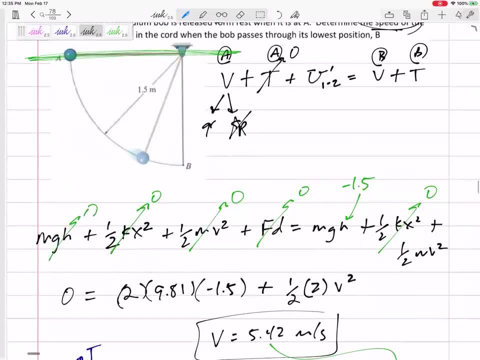 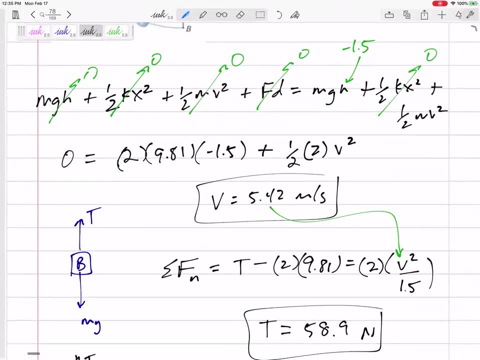 of asking for the speed, we use conservation of energy to find the velocity and we use free body diagram to find the force in the cable forcing the tension of the cable. Okay, let's jump back.